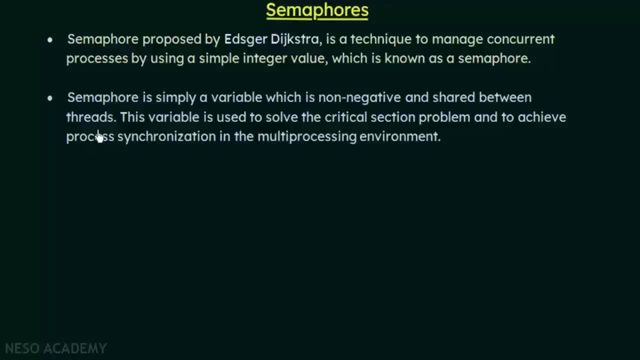 which is non-negative and shared between threats. this variable is used to solve the critical section problem and to achieve process synchronization in the multi-processing environment. so that is what i just said. semaphore is simply a non-negative integer value that is shared between threats, so it is a shared variable and this variable will be used to solve the 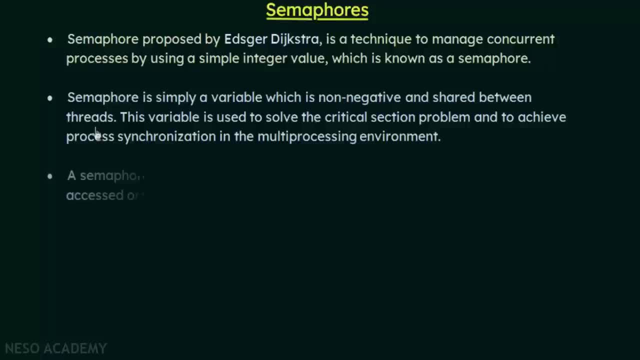 critical section problem, and how is it done? we will be seeing that. so a semaphore s is an integer variable that, apart from initialization, is accessed only through two standard atomic operations, which are called semaphore and. semaphore s is an integer variable that, apart from initialization, is accessed only through two standard atomic operations, which. 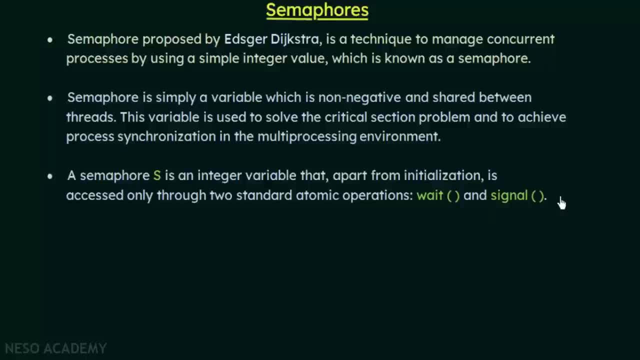 are weight and signal. so we understood that semaphore is an integer variable which is shared between different processes. now another thing is that this integer value s called the semaphore. it can be accessed by processes through only two standard atomic operations, which is known as the weight and signal operations. so whenever you study about semaphores, this weight and signal operations 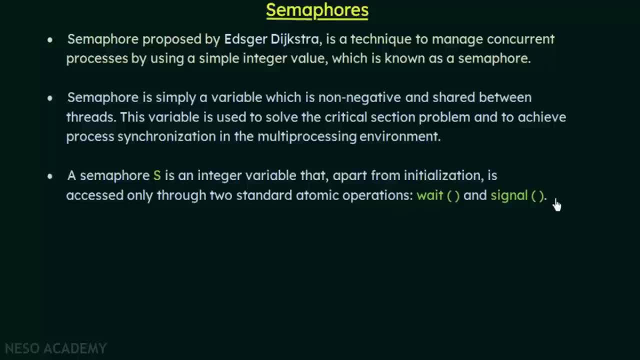 are two important things that you need to know about, so we'll be seeing what is this weight and signal operation? so, whenever you study about semaphores, this weight and signal operations are two important things that you need to know about, so we'll be seeing what is this weight and signal operations use for. 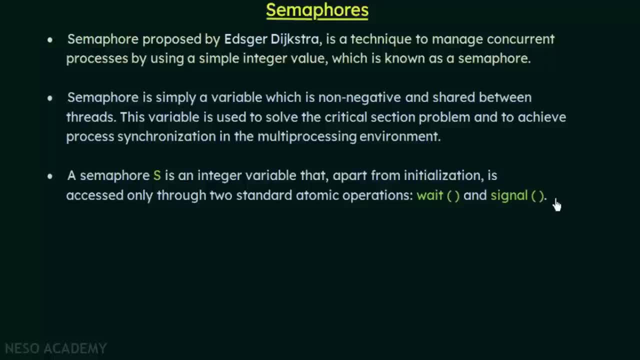 and how they are defined and how processes will be making use of these two operations to access semaphores. so before we go into the definition of weight and signal operations, let's first familiarize ourselves with the terminologies that are used to denote weight and signal. so weight is denoted by the letter p, which is derived from the 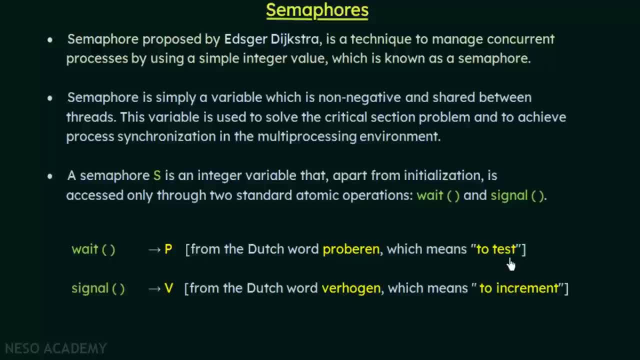 dutch word proberen, which means to test and signal, is denoted by the letter v, which is from the dutch word verogen, which means to increment. so whenever you study about weight and signal or read about this in books, you'll be seeing that they are denoted using the letters p. 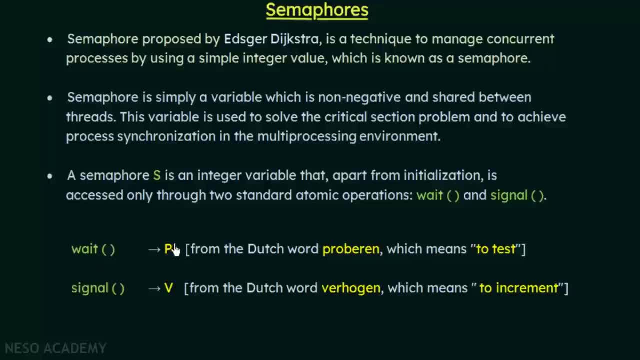 and v respectively. weight is denoted using p and signal operation is denoted using v. so where did this come from? this is what we just saw. they came from these dutch words. so p is taken from this word and v is taken from this word. and why is it dutch? because it's a dutch word. so it's a dutch word. so 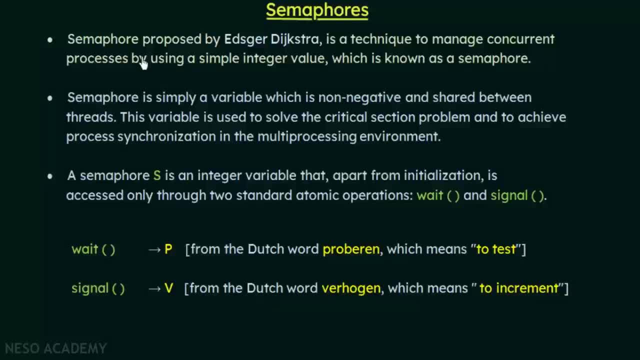 it's a dutch, because we know that the one who proposed this semaphores, that is, the computer scientist dystra, was from netherlands and he is a dutch man. so that is why probably he must have given these terms. so now we may be thinking: why did he give these letters p and v? why this word? 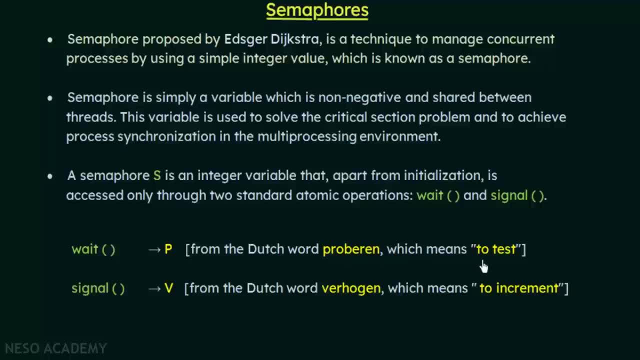 proberen and verogen, why does it mean to test and why does it mean to increment? so these two things we will be understanding when we look at the definition of the weight and signal operations and see how it is defined and how this will help us in process synchronization. so here, first of all, 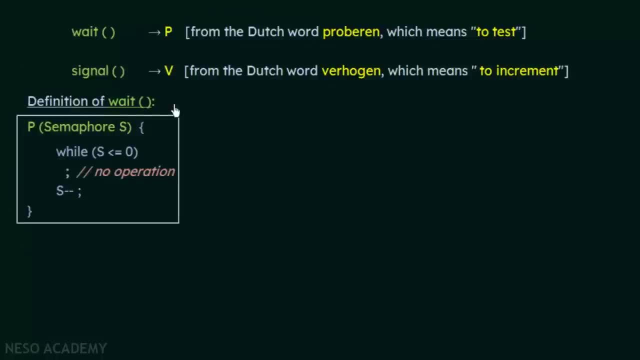 we'll be seeing the definition of the weight operation. so the weight operation is defined like this. so here, as i told you, p is used to denote the weight operation. so when the semaphore s needs to be accessed using the weight operation by a process, what happens is it will check whether 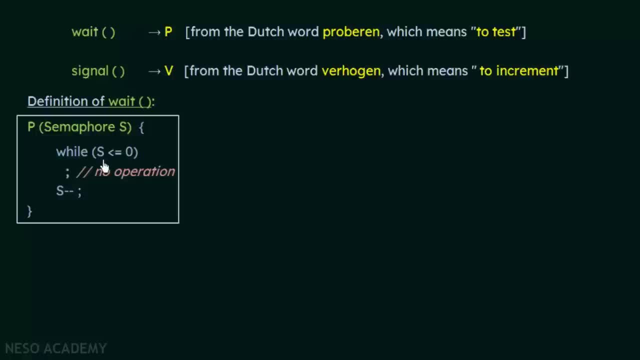 the variable s is less than or equal to the weight operation. as i told you before, this is also a way to zero. So let us recall that S is a semaphore, which is an integer variable that is shared between different processes, So it is a shared variable. So whenever I say S, know that. 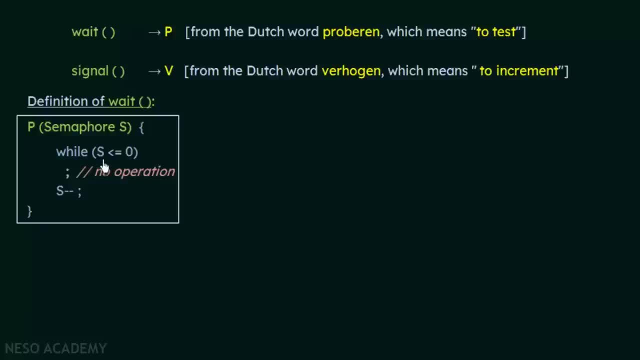 it is a semaphore. So it will first check. if the semaphore variable S is less than or equal to zero, Then we see that there is a semicolon here. So if there is a semicolon right after the while condition, what does it mean? It means that there are no operations. 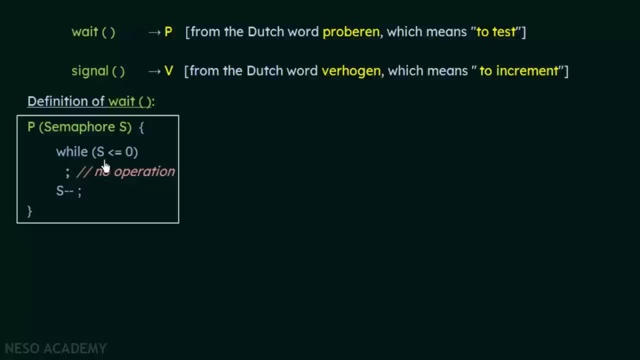 under this while loop. but as long as the condition is true, the control will be stuck inside this while loop looping as long as this condition becomes false. So if S is less than or equal to zero, it will stay inside this while loop and it will never come out. 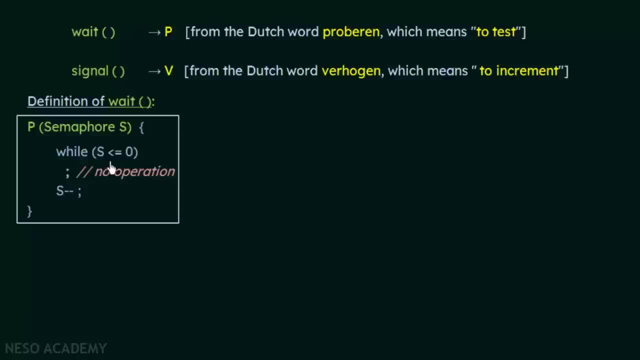 of this while loop. But if S is not less than or equal to zero- that means, if S is greater than zero- then what happens? It will break out of this while loop and it will decrement the value of S. So that is what happens in the wait operation. Now what does this all signify? So here: 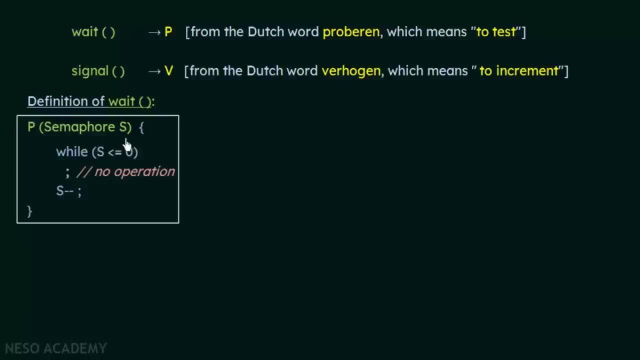 what happens is that, as I told you, S is a semaphore variable that is going to be shared between processes. So when one process wants to, let's say, access a resource, or let's say that it wants to enter this critical section, So at that time this variable, S, that is. 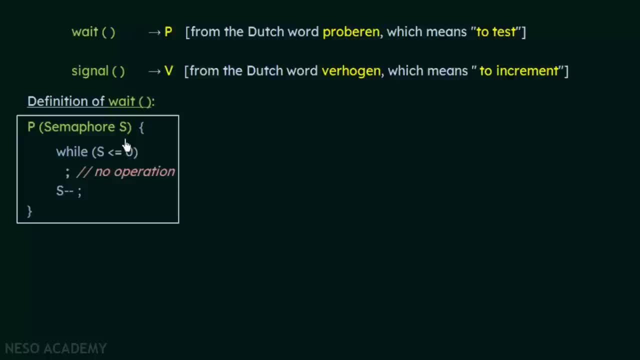 shared between the processes will take care of who should access the resource or who should enter the critical section. So if the value of the semaphore S is less than or equal to zero, that means that some process is already making use of the shared resource or is already there in the critical. 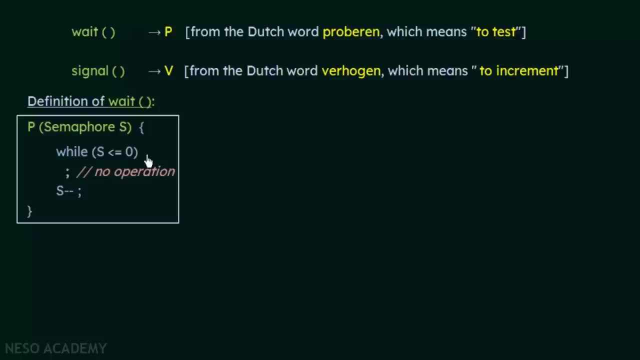 section. So at that time no other process should be allowed to enter the critical section or it should not be allowed to use the resource that is being shared. So that is why, when the process wants to access the shared resource or wants to enter, 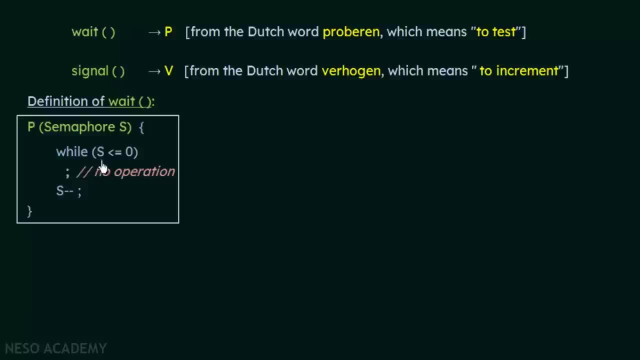 the critical section. it will check this condition and while checking this condition, if this condition is true, the semaphore S is not allowed to enter the critical section. So then it will be stuck here and it will not be allowed to enter the critical section, or it will. 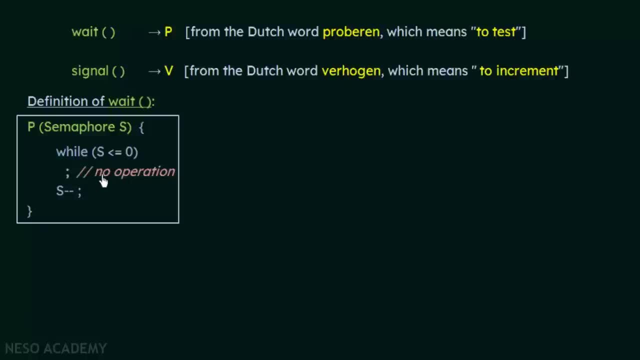 not be allowed to use a shared resource. So that is what happens here. Now, if this condition is not true- that means if the value of s is greater than 0, then what will happen? Process will not be stuck in this loop, but it will come out of this loop and decrement the value of s and enter. 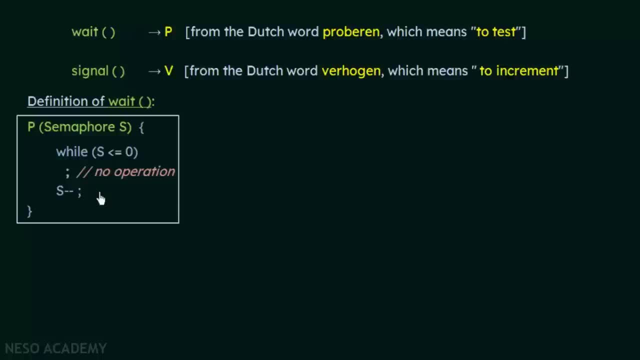 the critical section or make use of the resource that it wants to use. Now, why is it decrementing the value of s? It is decrementing the value of s because it needs to let other processes know that the semaphore's value is now decremented. Hence, when some other process wants to enter the critical 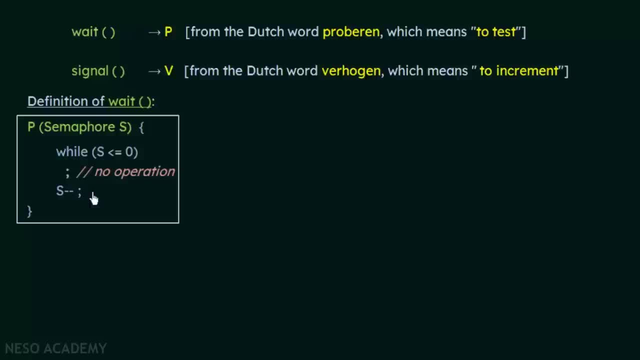 section or wants to access the resource based on this decremented value, the condition will either be true or false for that process. So that is why this decrement of semaphore is done over here. So again, there are two types of semaphores which we'll be discussing. So, based on those two types, 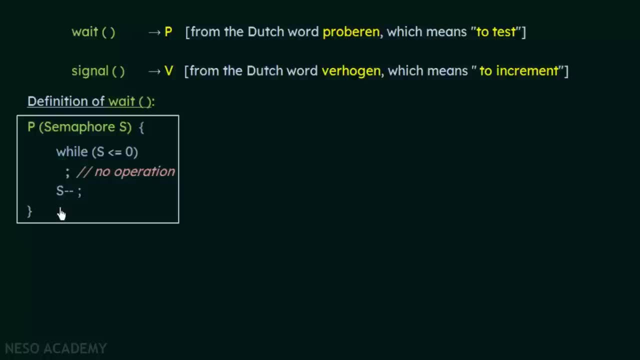 of semaphores. when we explain it, this will become clearer. Alright, so remember that this wait operation is used to test if there is any other process using the resource or if any other process is there in the critical section, and if it is not there, it will decrement and enter the critical section, or 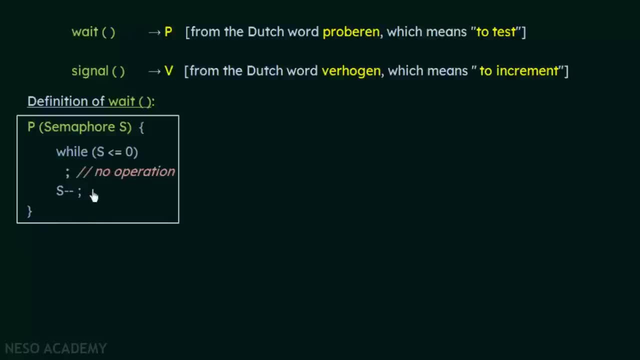 use the resource, or if some process is already using the resource or is already in the critical section, this while condition will be true and the requesting process will be stuck here. So this wait is actually used for testing. So that is why this word probaren is used, which means to test. So that is the definition of the wait. 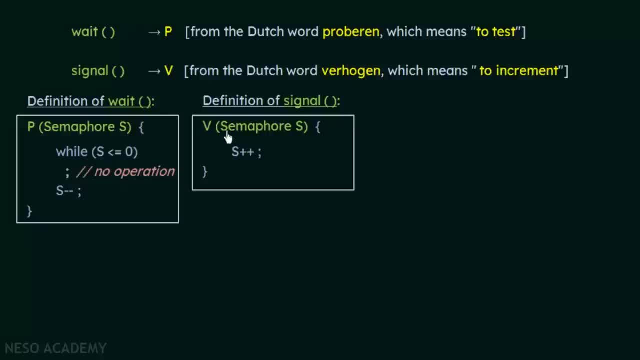 operation. Now let's see the definition of the signal operation. In the signal operation it is nothing. it just increments the value of s. So this signal operation will be called when the process that was making use of the semaphore to enter its critical section or was using a resource. 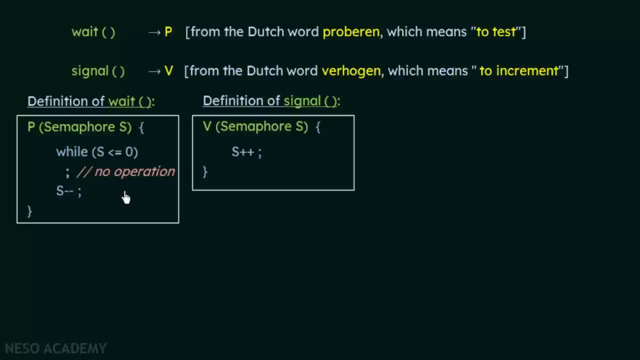 completes its operation and comes out of it. So here we see that there was a decrement operation. Now, when the process enters its critical section or has used the resource that it wanted to use by making use of this wait and coming out of this while loop, at the end it has to again increment. 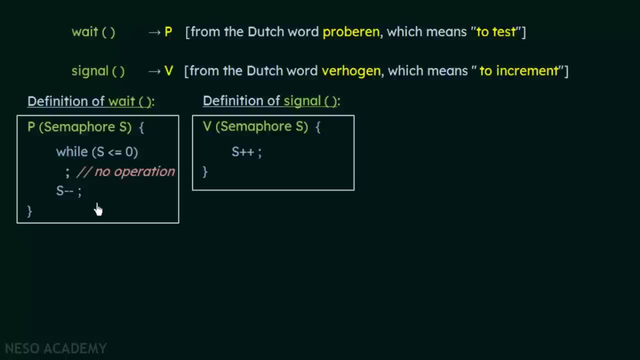 the value of s, Hence denoting that it has now released the semaphore. So that is why this increment operation of s is happening here. So signal will be used by a process to signal other processes that I have completed using the semaphore, and if you want to use it, you are free to use it. 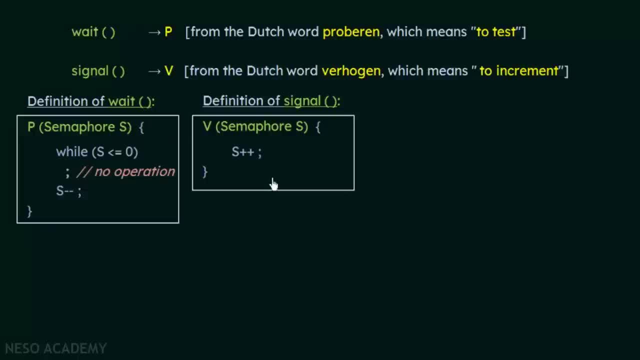 So that is what we are going to do here. So let's see the definition of the semaphore. So that is meant by this signal operation. So those were the definitions of the wait and signal operations. Now, another thing that we have to keep in mind, which is very important, is that all the modifications 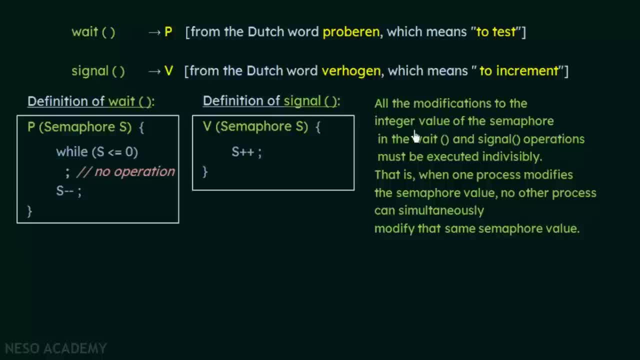 to the integer value of the semaphore in the wait and signal operations must be executed indivisibly. What does that mean? That means that when 1 process modifies the semaphore value, no other processes can simultaneously modify that same semaphore value. So, as I already told you, the semaphore variable. 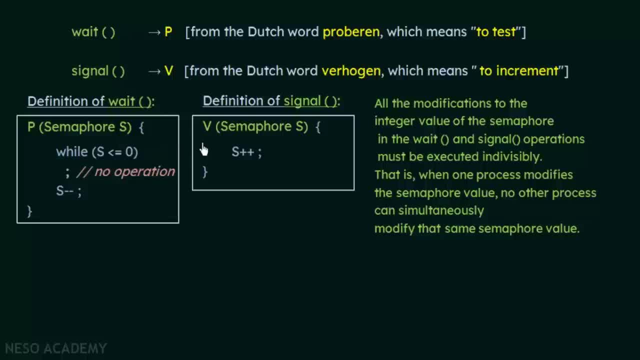 s is shared between the different processes, so when one process is modifying the semaphore value, then no other process can modify its value until and unless it completed its modification. so here we see that there are certain modifications happening, like, for example, here s minus minus: there is a decrement happening. here there is s plus plus: there is an increment happening. so 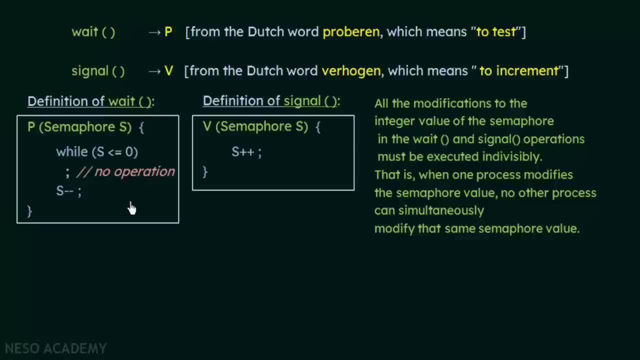 these are examples of where the semaphore's value is modified. so when one process is modifying the semaphore, then no other process should modify the semaphore at that particular instant of time. so that is what we mean by this. it is an indivisible operation. all right now, as i told you, there are 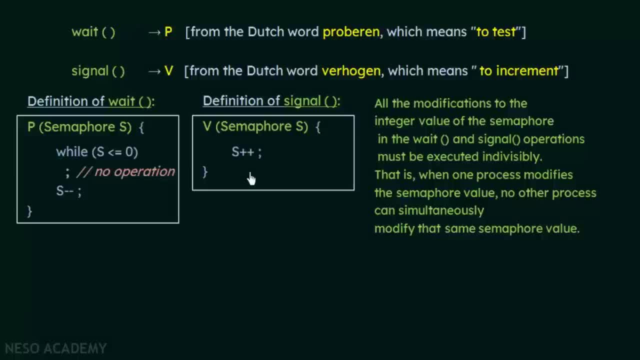 again two types of semaphores that we have. so we'll be seeing what are those two types and, based on those two types, we'll be trying to explain this weight and signal operations again, which will make it clearer to us. so, coming to the type of semaphores, we have two types and then the first. 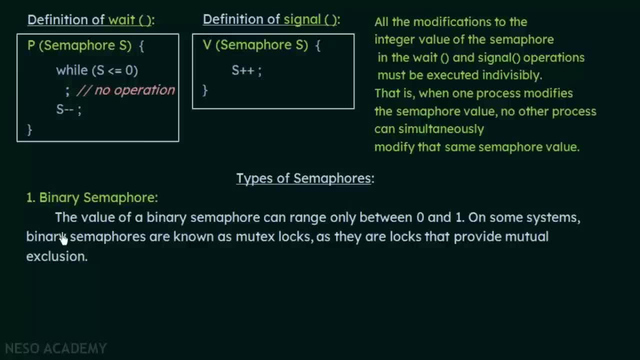 type is binary semaphore, so the value of a binary semaphore can range only between zero and one. on some systems binary semaphores are known as mutex logs, as they are logs that provide mutual exclusion. so this is the first type of semaphore. so from the name itself we can understand that binary. that means the value of. 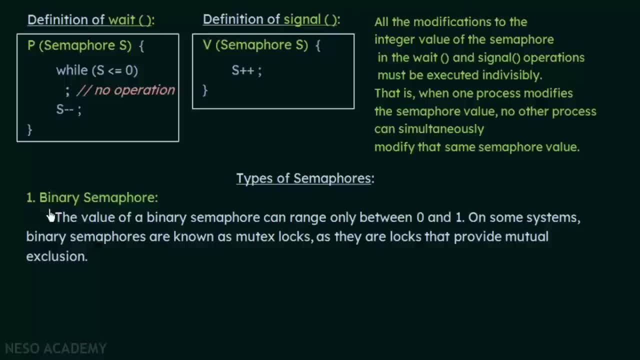 this binary semaphore can only have two values, which will be either zero or one, and on some systems, these binary semaphores are known as mutex locks, because they are the logs that are used to provide mutual exclusion. and how is it? we'll see that. so let's come back to the definition of 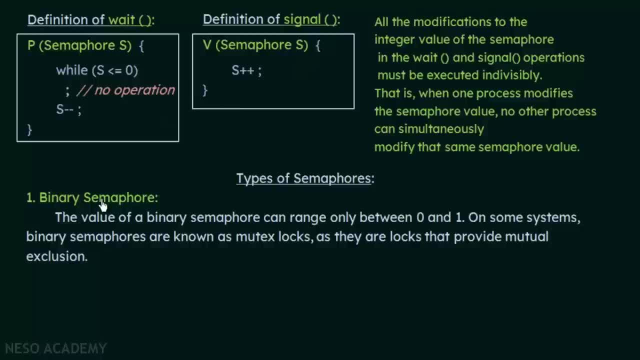 weight and signal, and try to explain this on the basis of binary semaphores. so, as i told you, it will have only two values, either zero or one. so if the value is zero, that means that the shared resource is being used by some other process and the currently requesting process has to wait, or 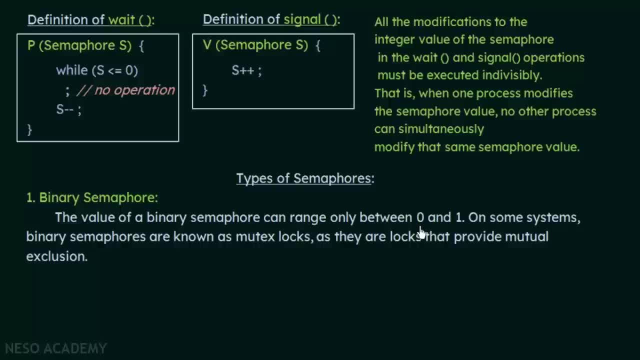 if we talk in terms of critical section, if s has the value zero, that means that some process is already executing in its critical section and the requesting process has to wait, and if the value of the semaphore is one means that it is free for the currently requesting process to either enter this critical section or to use the shared 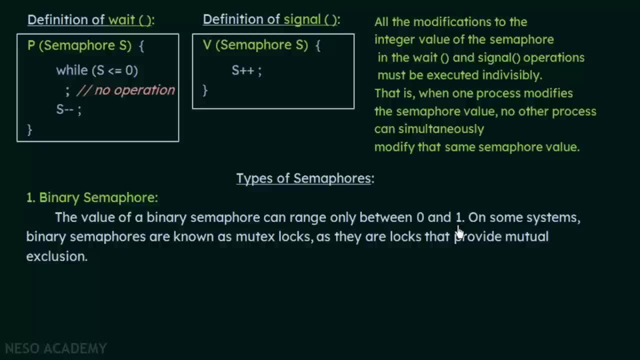 resource that it wants to use. so let's see, let's take two cases. so in the first case, let's say that there is a process that wants to either enter this critical section or wants to access a shared resource. so let's say that there is only one shared resource and that 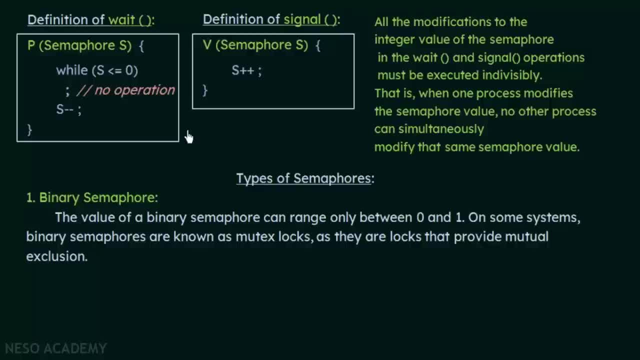 shared between different processes. So let's say that in this first scenario, the resource is not being held by any other process right now. Or if we talk in term of critical section, let's say that the critical section is right now free. No other processes are executing in their critical. 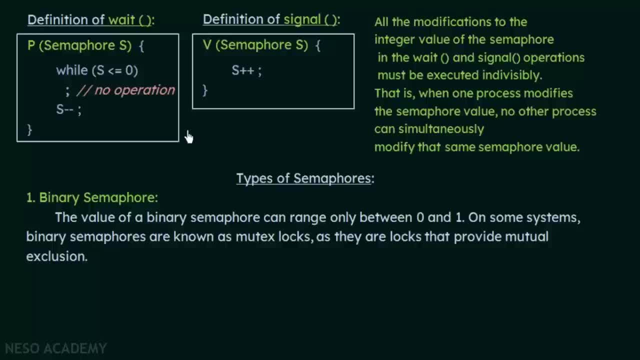 sections, and the process that wants to currently execute in the critical section is free to do so. So remember one thing: that the value of semaphore will initially be initialized to the value 1.. So 1 will be the initial value of the semaphore. So what will happen? The process that wants to 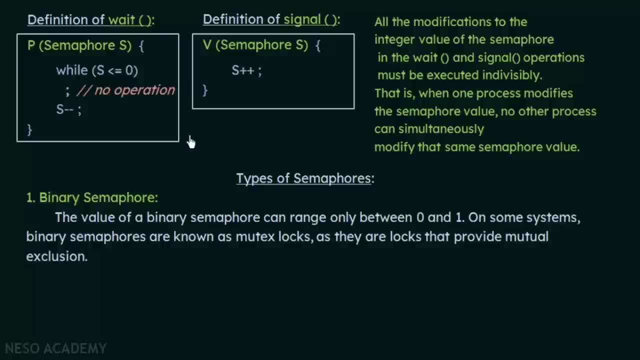 access the shared resource or enter its critical section, will come and access the semaphore through the wait operation. So in the wait operation, that is P, what will happen? Here? we have the semaphore S and, as I told you, right now, in this scenario, we are assuming that no other processes are there. 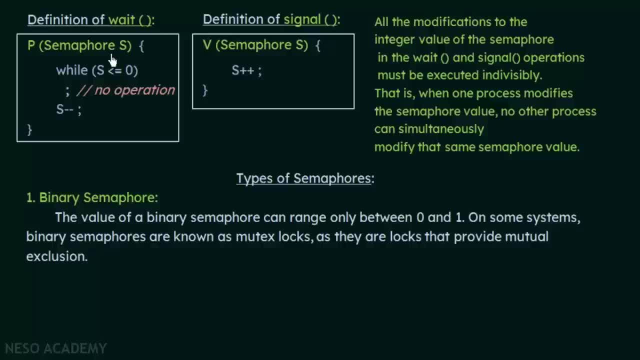 in the critical section or no other processes are using the shared resource. So the value of the semaphore is 1.. So it comes to this while loop and checks the condition. If S is less than or equal to 0, the condition is false because, as I said, the initial value of S is 1. So it does not enter. 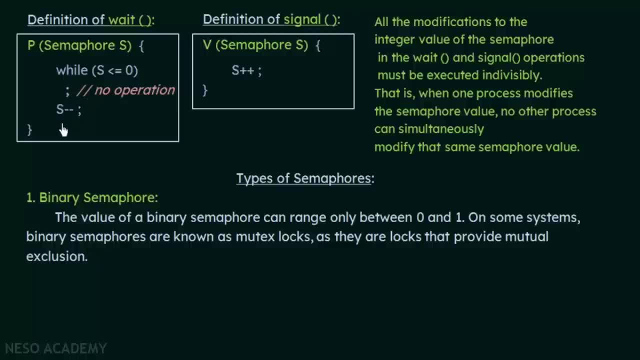 this while loop. but it breaks from the while loop and it comes here where it says S minus minus. So that means decrement the value of S. So what was the value of S? I told you. it is initialized to 1 and then it will decrement the value of S, making it 0. now, 1 minus 1 is 0, and then it will. 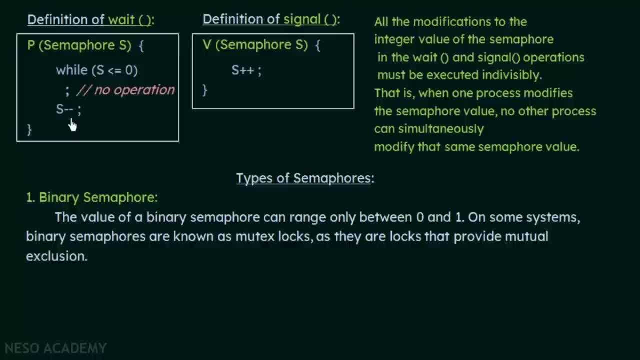 either enter the value of S or it will enter the value of S. So it will enter the value of S. so if S is less than or equal to 0,, then it does not enter the critical section or use the shared resource that it wants to use. Alright, So when that process is now executing, let's say that 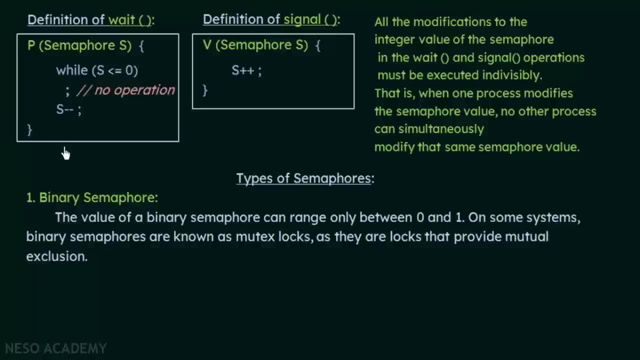 there is another process coming now, scenario 2. There is another process that wants to enter its critical section, or let's say that it wants to use the shared resource. So what will happen? That process will also come and access the semaphore through the wait operation. So when? 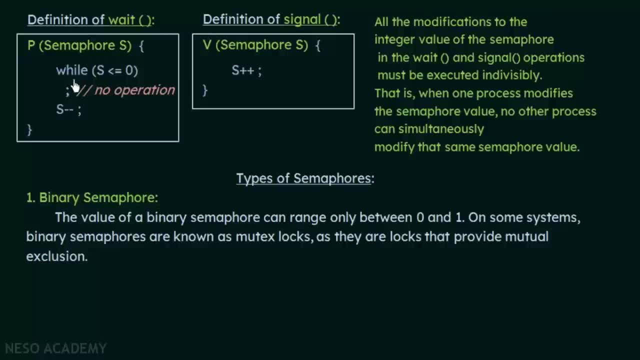 it accesses the wait operation, what happens? It will check this condition again. Is S less than not equal to 0.. So we saw that the final value of s was equal to 0. The previous process already decremented and made it 0. So this condition becomes true: s is equal to 0. So when s is 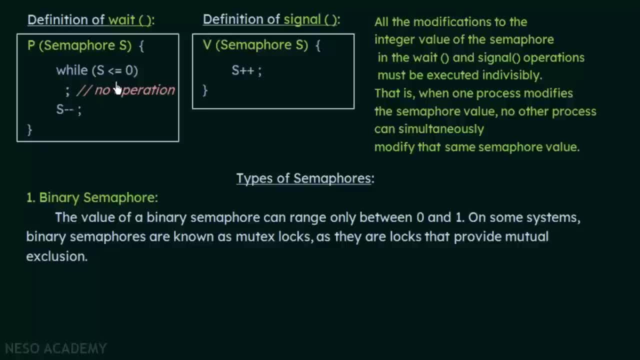 equal to 0,. what happens? That process will not be able to come out of this while loop. It will be stuck in this while loop and it will not be able to come out of it, and hence it will not be able to enter its critical section, or it will also not be able to use the shared resource that it wants. 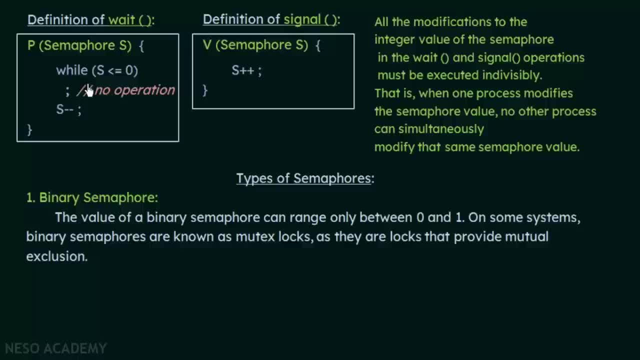 to use. So it gets stuck there. Alright, now let's come back to scenario 1, where the first process was able to enter the critical section or access the shared resource and it was using it. and let's say that it now completes using the shared resource or it is now exiting from its. 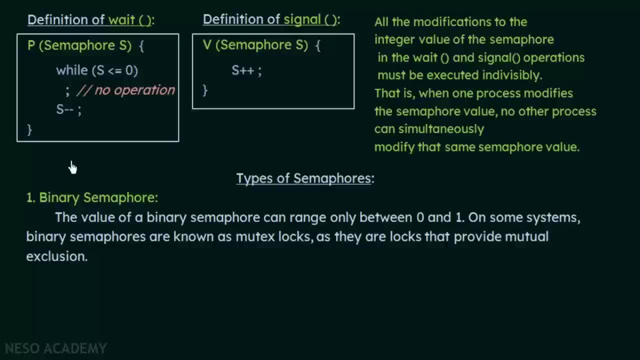 critical section. So, at that time, what will it do? It will call the signal function or the signal operation. So it will call the signal operation and it will increment the value of s, s++. So now, what will be the value? 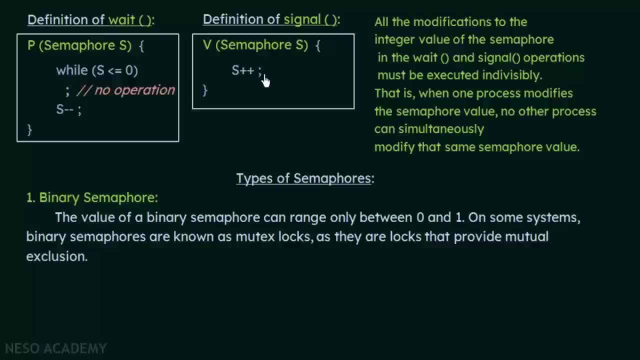 The value of s. we know that s value was 0.. Now, when it does this increment, operation, s value will be incremented by 1.. Hence it will become 0 plus 1, equal to 1.. So the value of s is now 1.. What does? 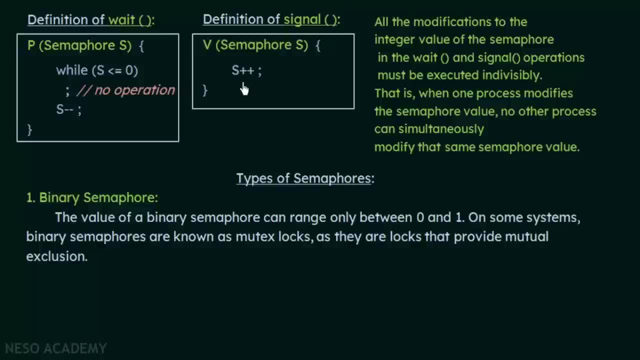 that mean? That means that this process is signaling other processes that I have completed using the critical section or the shared resource, whatever it may be- and the semaphore can now be used by some other process. Now, in scenario 2, we saw that there was one process that 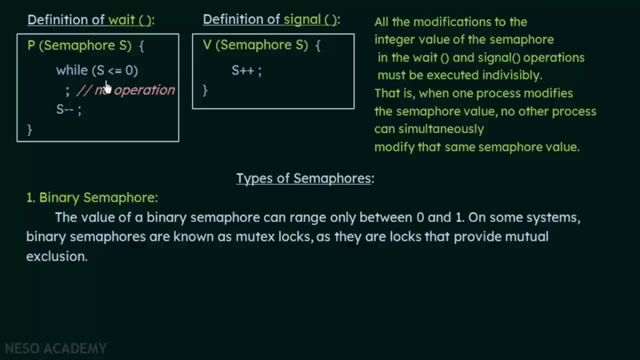 was trying to access the critical section or shared resource, but was not able to do so because this while condition was true. But when the first process increments the value of s, now what happens? The value of s becomes 1.. This condition will now become false. The process that was stuck. 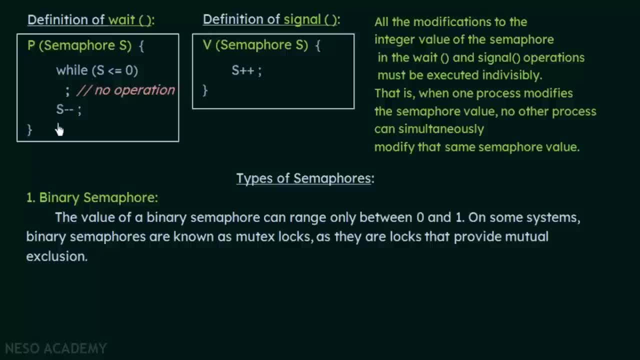 in this loop, will break out of this loop, and what will it do? It will now decrement the value of s by itself. So what was the value of s? It was 1, and now that process will decrement the value of s, making it 0.. 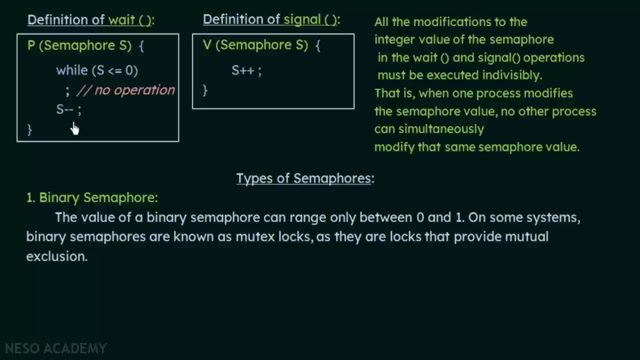 So when the semaphore is running, it will enter its own critical section or access the shared resource that it wants to access. So that is how it happens. and again, when that process completes its execution, it will access the signal operation and increment the value of s. So that is how. 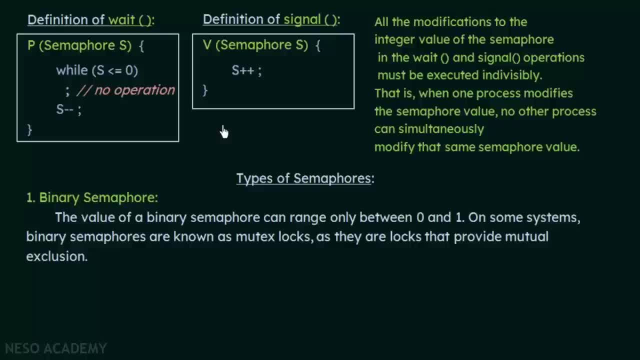 binary semaphores work, We saw that there are only two values, either 0 or 1.. So when it is 0, that means that some process is already making use of the semaphore, and it is either executing in its critical section or using the shared resource. 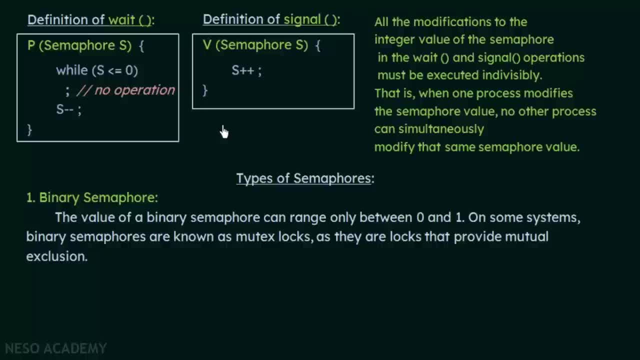 processes can use it. We saw how it works. and if the value is not equal to 0, that means if it is 1, then the process is free to use the semaphore and it can enter its critical section or use the shared variable. Alright, so that is how binary semaphores work Now. 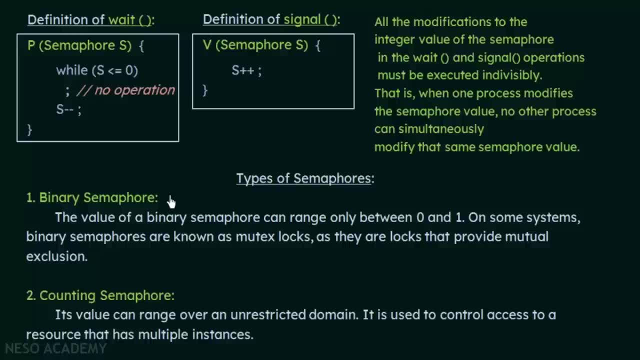 let's go to the next type of semaphore. So the next type of semaphore that we have is counting semaphore. Its value can range over an unrestricted domain. It is used to control access to resource that has multiple instances, So, unlike binary semaphores where it could. 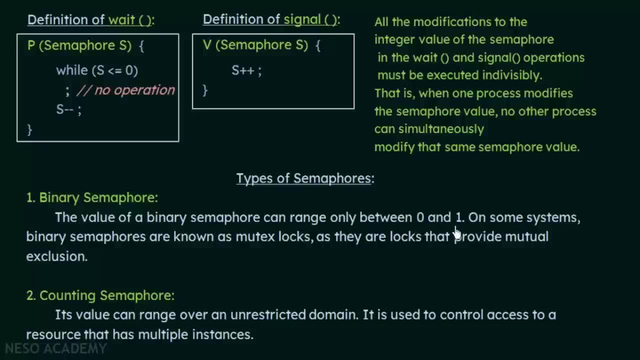 have only values of 0 and 1, in counting semaphore, it can have a range of values that will range over an unrestricted domain. That means it can have multiple values. It can be 1,, 2,, 3,, 4, so on. So why is this used? This is used to control access to resources that has 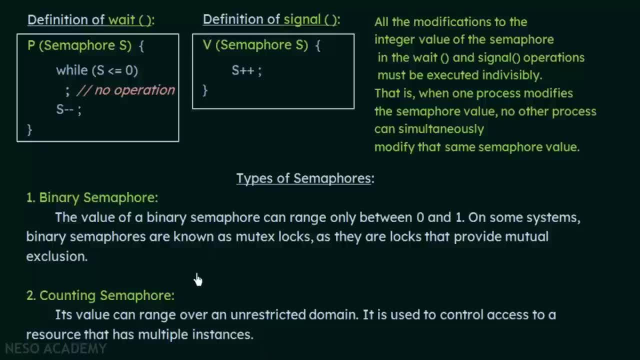 multiple instances. So let's say that there are several processes that are sharing a particular resource. So let's say that there are three processes. So let's say that there are three processes: P1, P2 and P3.. Let's say that their resource is having multiple instances: R1 and R2.. That 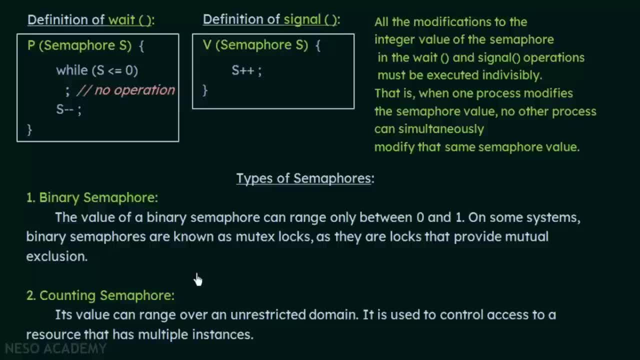 means it is not just one resource, but that same resource is having multiple instances, so multiple processes can make use of it. So P1 can use resource R1 and P2 can use resource R2.. So in that way, if there are multiple instances of a particular resource, 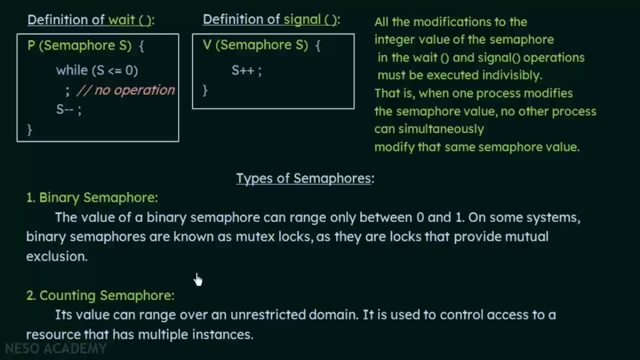 then multiple processes can make use of it. But again, it is limited. The resource will not have indefinite or infinite instances. So in order to control that, we are going to make use of this counting semaphore. So again, let's take this example of the weight and signal. So let's say that 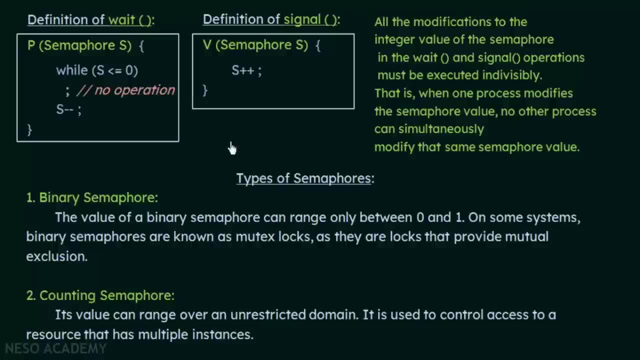 there are processes P1, P2 and P3, and there is a resource which is having two instances. That means that the resource can be used by two processes at the same time because there are two instances of the same resource. So we will set the value of our counting semaphore. 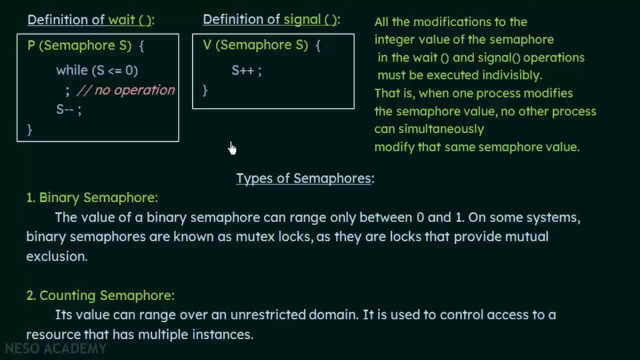 equal to 2.. So 2 is the number of instances that are resources having. So again, let's say that we are assuming that the resource is not being used by any processes at this moment, And so the S value, that is the semaphore value, 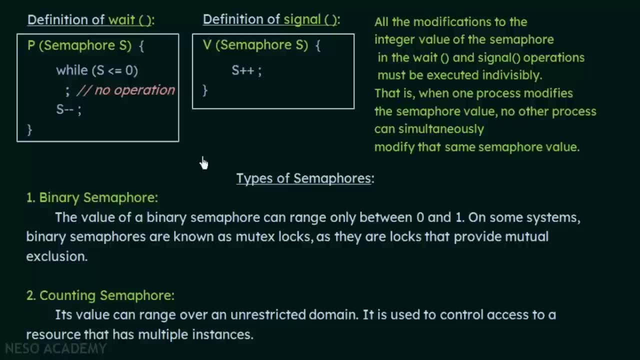 will be 2.. So now let's say that a process- P1- wants to make use of the resource. So what will happen? It will come to this weight operation and it will check for this, while condition Is S less than or equal to 0? What is the value of S? It is 2 because we have 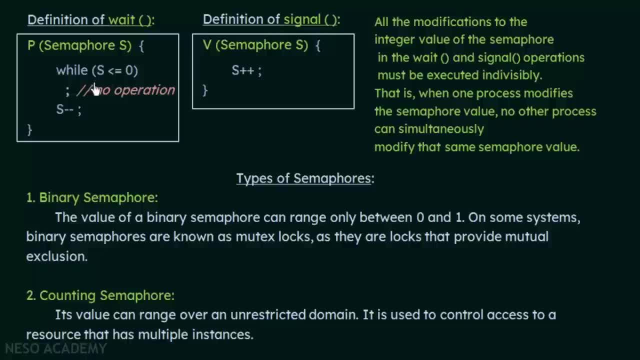 two instances of the resource. So is this while condition true? It is not true. So it will not come to this while condition and it will just decrement the value of S. Now the value of S was 2, it decrements and makes it 1, and then that process will use the resource. 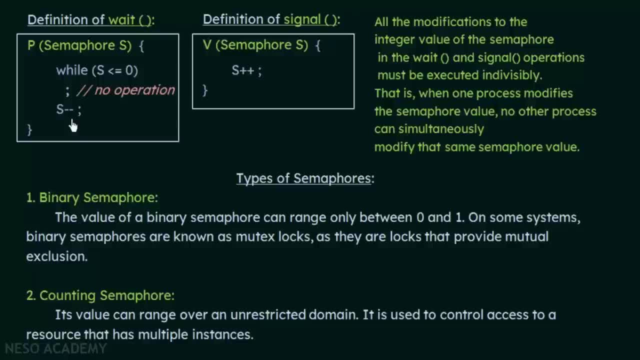 that it wants to use. Now let's say that at this time there is another process, P2, that arrives and P2 also wants to use the same resource. Now, as I told you, there are two instances and one instance, as we saw, is already taken by process P1.. Now, if P2 wants, 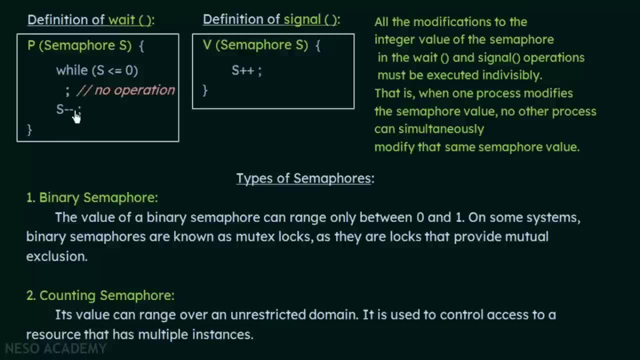 to access the same resource. what will happen? It will also come and execute this weight operation And here it checks: is S less than or equal to 0?? What is the value of S? The value of S is now 1, I told you, because it was decremented here. So again, this condition becomes false. 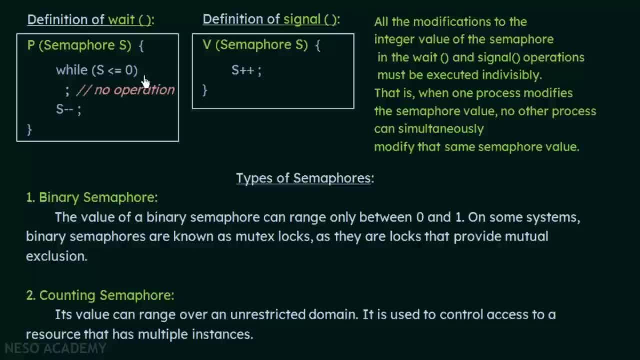 because S is not less than or equal to 0. So it will also not enter this while loop, but it will break from here and it will decrement the value of S and will make use of the resource Now, when it decrements the value of S. what is the value of S now? The value of S will. 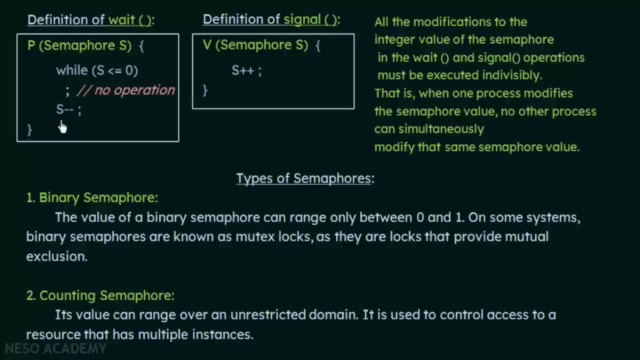 now become 0. It was 1.. So once it decrements here it will become 0. So it will also make use of the resource. Now we see that there were two instances of the resource and both are now used by two processes: P1 and P2.. Now let's say that there 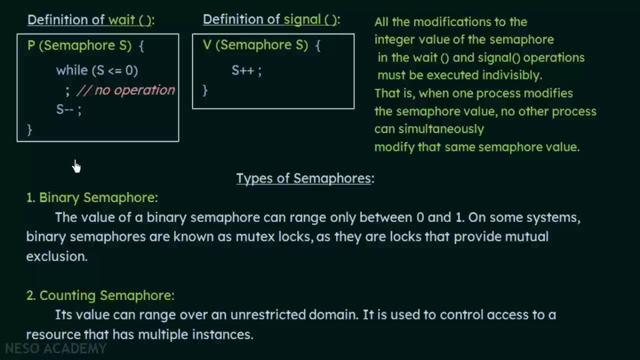 is another process that arrives P3,, which also wants to make use of the same resource. So it will also make use of this weight operation and it will check here if S is less than or equal to 0.. So now this condition becomes true. We know that both the instances of the 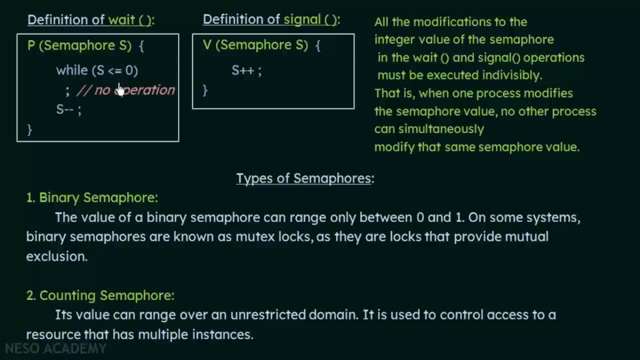 resources are being used by processes P1 and P2.. So now the value of S is 0. We already saw why it is 0. So this condition becomes true. So process P3 will get stuck in this loop because this condition is true, and it will. 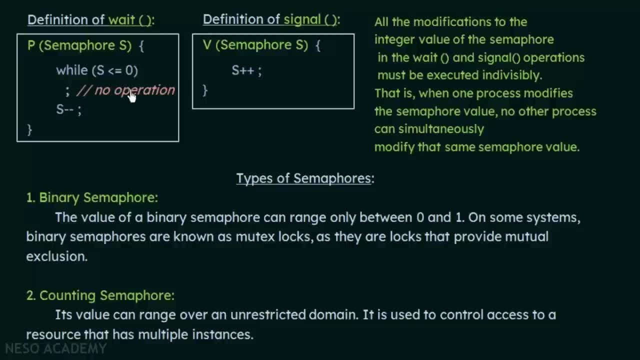 get stuck in this loop, and it will remain in this loop as long as this condition doesn't become false. Now let's say that one of the processes from process P1 or P2, one of them, completed using the resource, and then, when it completes using the resource, what will? 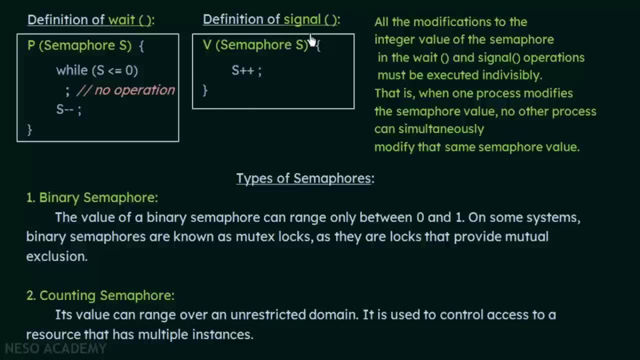 happen, It will call the signal operation. So while calling the signal operation, it will increment the value of S again. So the value of S will become 1 now From 0, it becomes 1 because of this increment. So that shows that the resource is now released by process. 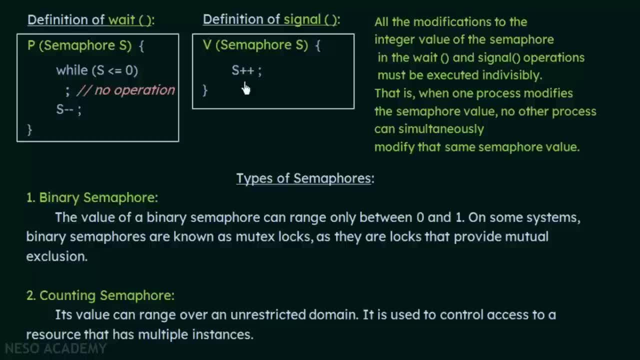 P1 and it is available for other processes to use, And here we see that there was one process trying to use it which was stuck in this loop. So when process P1 increments its value of S, what will happen? This condition will now become false. S is less than or equal. 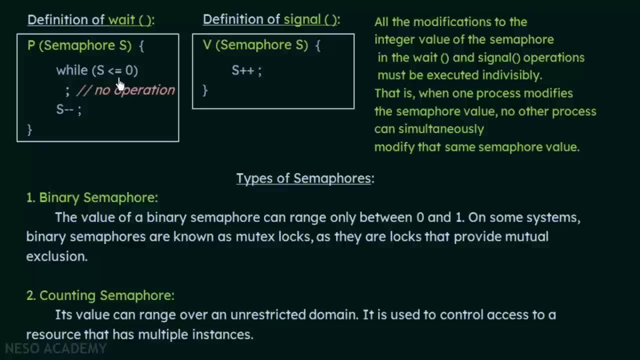 to 0. It is false now because S value is now 1.. It will break from this loop and it will also decrement the value of S and will be able to make use of the resource. So that is how the counting semaphore works. It is not just. 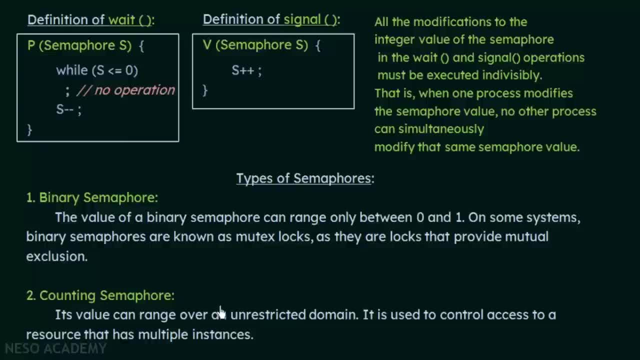 ranging between 0 and 1, but it will have a range within an unrestricted domain depending upon the resources that we have. So if we are having resources having multiple instances, we can make use of counting semaphores. So, as long as the instances of resources are. 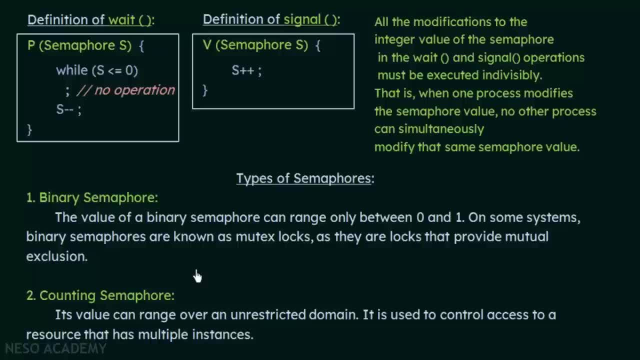 available, the processes will be able to use them. But once they are not available, we can use them. So in this case, we have run out of resources. Once we have run out of resources, then the other processes will not be able to access that particular resource.